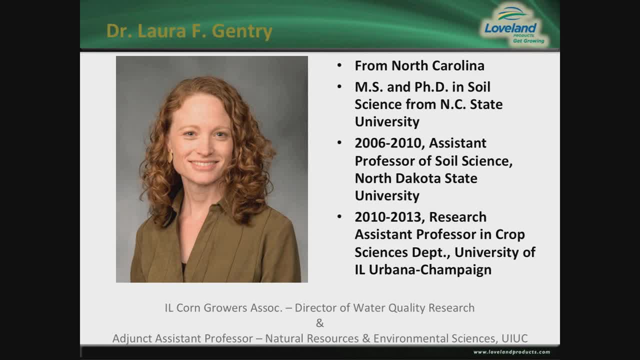 at North Dakota State University. She received her master's and PhD in soil science from North Carolina State and she is originally from North Carolina. She resides on the Illinois Corn Growers Association as a director of water quality and research and she's an adjunct. 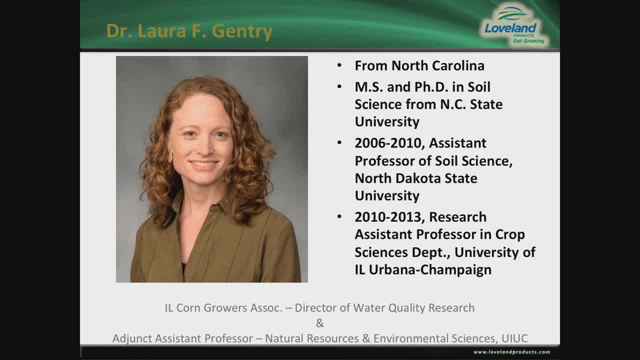 assistant professor of natural resources and environmental sciences at the University of Illinois, Urbana-Champaign. So, without any further ado, we're going to allow Dr Gentry to give her presentation and then I'll be back After that with some more information about this technology. 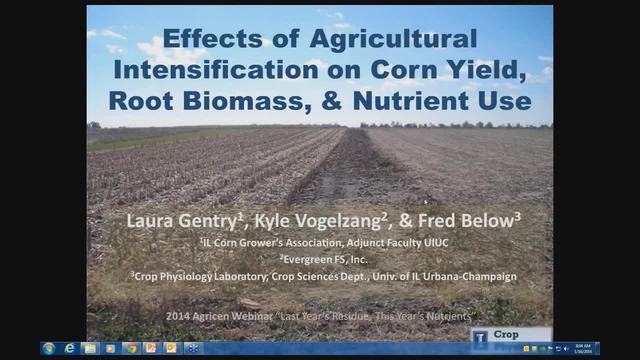 I thank you all very much for giving me this opportunity to share a little bit of the research that we're doing in the crop physiology lab at the University of Illinois, and especially what we're doing in regards to stover removal and nutrient management in continuous corn. 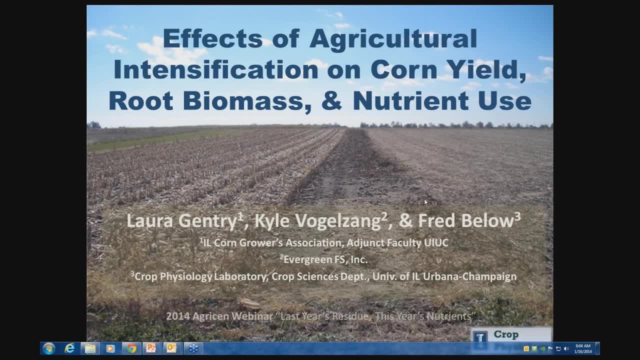 systems, And I'd like to start by acknowledging my co-authors, Mr Kyle Vogelzang and Dr Fred Bilo. Kyle was a graduate student. He was working in this research project with us and he was responsible for 100% of all. 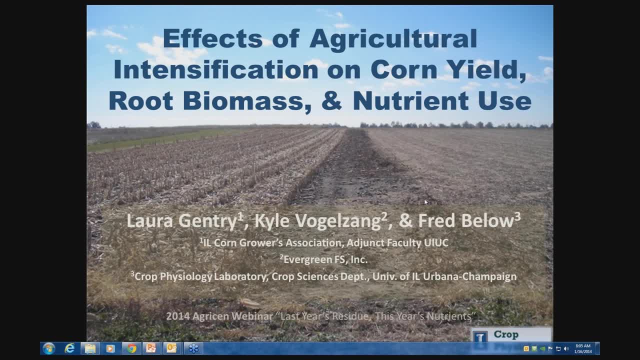 of the roots that were dug during the course of this project, And that was a thankless, dirty, arduous job, And he was also instrumental in managing this study and implementing a lot of the treatments for it, And so now Kyle is working at Evergreen FS in Evergreen Illinois. 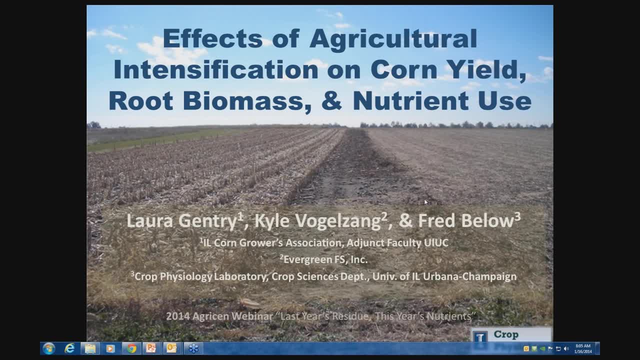 as a crop consultant. Dr Fred Bilo is a Professor of Natural Resources and Environmental Resources at the University, is a professor of Crop Physiology in the Crop Sciences Department at the University of Illinois, And Fred is the head of the Crop Physiology Lab here at the U of I and he was the person who 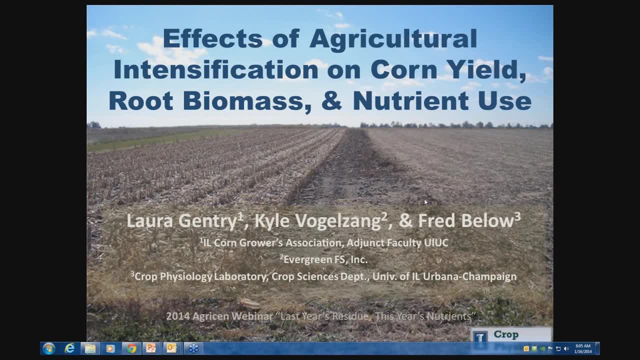 actually originated. the original project that this study that I'm presenting today was based on, or was sort of a follow-up to The original study, was initiated in 2003,, and it was an investigation of the causes of reduced yields in the continuous corn system compared to corn following a soybean. 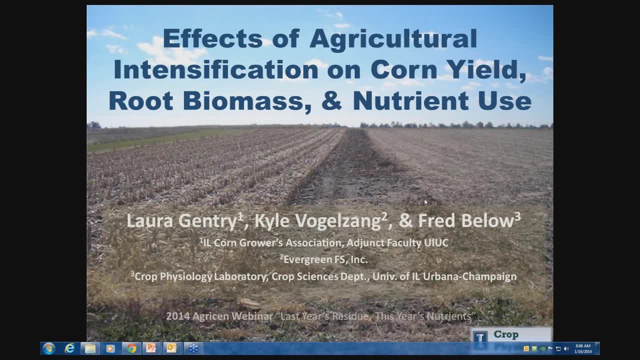 crop And we refer to that difference between continuous corn yields and corn following soybean yields as the continuous corn yield penalty And it's usually about 15 or 20, 25 bushels per acre throughout most of the corn belt. It varies but that's usually a pretty good estimate And that's. 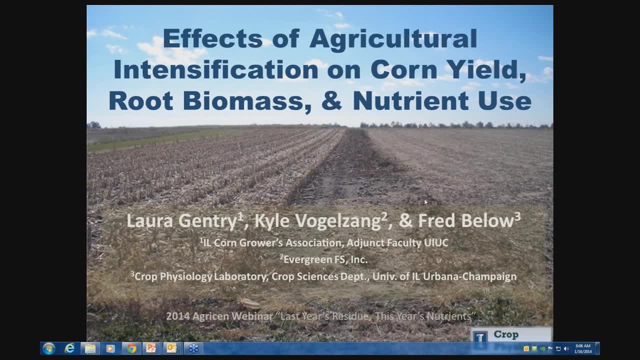 the difference between what you would see in a continuous corn system versus a corn following soybean- Kelly Runyon, 007, 007- And we want to to better understand that. So we established these large long-term blocks of continuous corn and corn-following soybean. That is also what this new study that I'm presenting today. 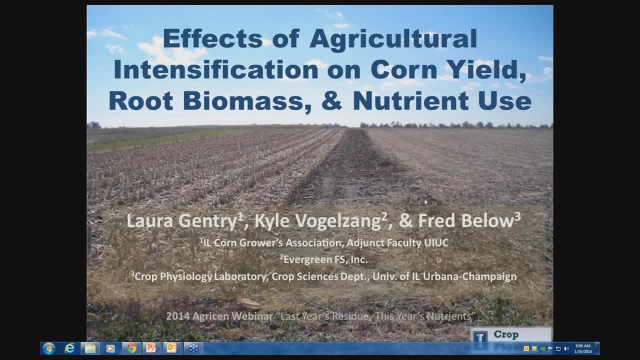 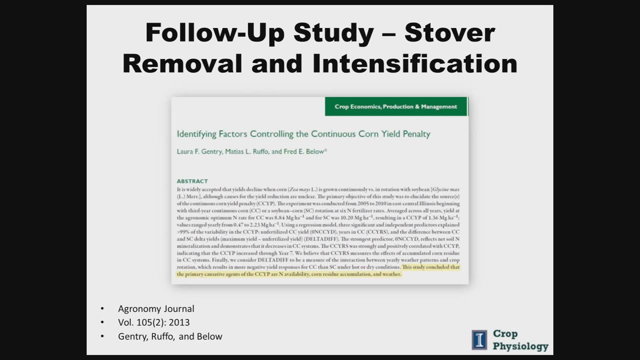 we went right back into those same plots to continue on the study to look at the effects of stover removal and nutrient use. This original study, the first one where we were just investigating what's causing the continuous corn yield penalty that we published in the agronomy- 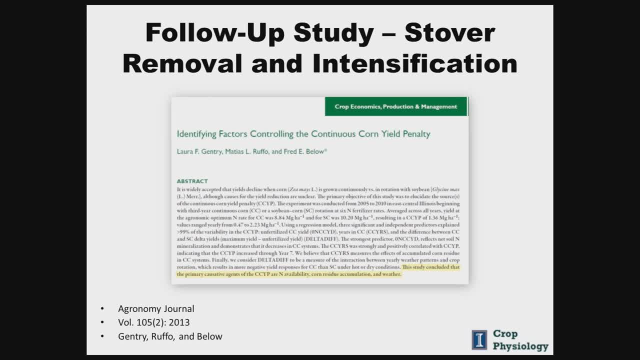 journal last year. it was myself and Fred Bilo and Dr Matthias Rufo, who now works at Mosaic Fertilizers, but he was a postdoc on this research project. In that analysis of our data we produced a model and that model determined that there were essentially three. 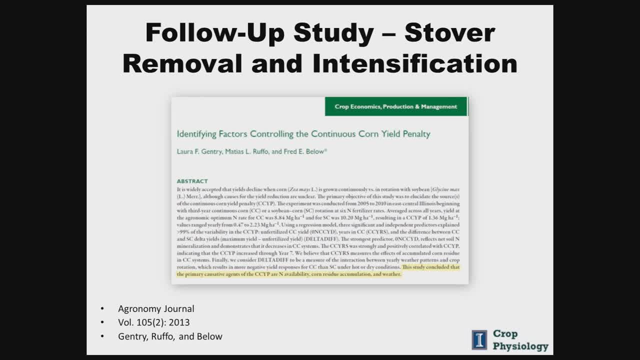 main factors that are causing yields to be lower in continuous corn systems relative to corn-following soybean. You can see that I highlighted here in this last sentence. here are the three factors that are causing yields to be lower in continuous corn systems relative to corn-following soybean. You can see that I highlighted here in this last sentence here. 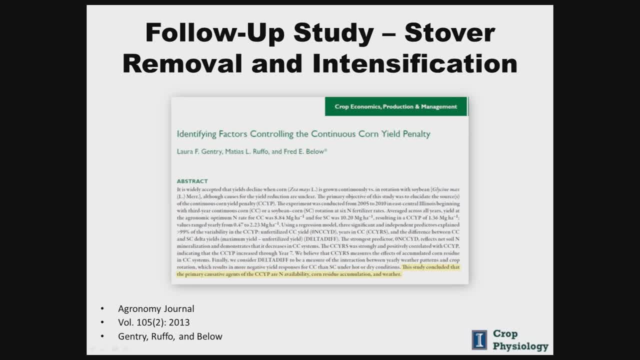 here the summary of that, which was that the three agents that are the major factors causing the continuous corn yield penalty are reduced nitrogen in continuous corn systems, and that's really talking about the mobilization of nitrogen by the corn stover, which has that high carbon. 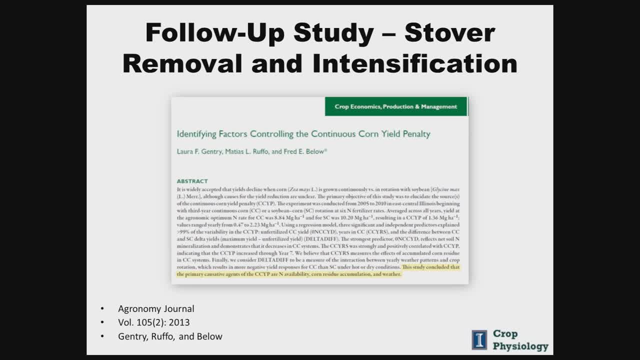 to nitrogen ratio. The second factor was all the buildup over the years of corn after corn, that stover can build up to a significant level and that residue has biological, chemical and physical factors that all combine together to reduce yields in continuous corn systems relative. 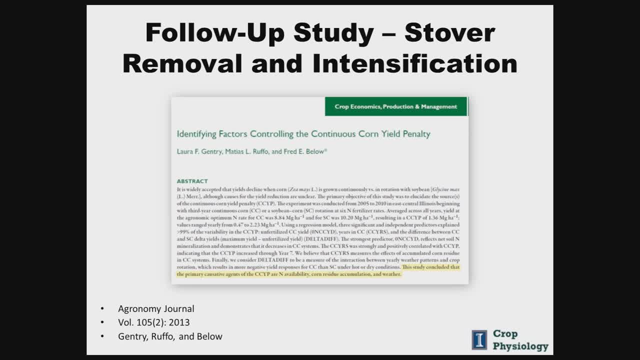 to a corn following soybean or another crop. And then the last factor was weather, and especially what we found was that the continuous corn system is not as resilient to drought, especially as is a corn following soybean, So the yields are going to be lower and the yield is going to be lower. 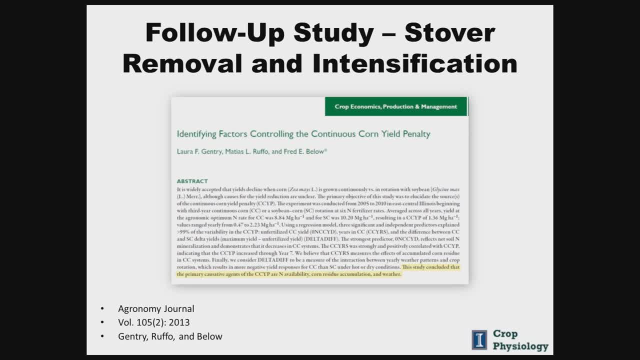 and they're going to be more detrimentally affected in a continuous corn system than they would be in a corn following a soybean crop if we have a really bad drought. So those were the three factors that we found, and we know we can't control the weather. the third factor, As far as the nitrogen availability. 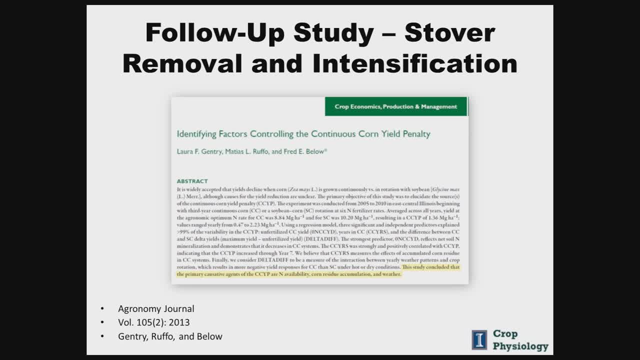 and the nitrogen mineralization. there are some new innovative products, such as the Agrison products, the Accomplish LM in particular, that do address nitrogen availability and they do address nitrogen mineralization in a really unique way with their biological products. We in this follow-up study, 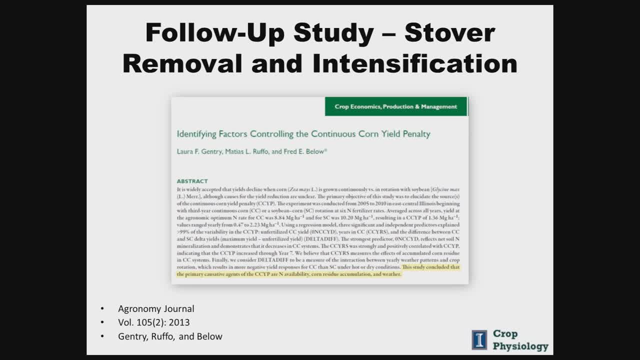 were really more interested in looking at the corn directly, looking at corn residue accumulation, and so we wanted to see what happens if we just remove some of that residue. And so our hypothesis for this study was that if we removed part of the stover, in our instance we removed 50% of the 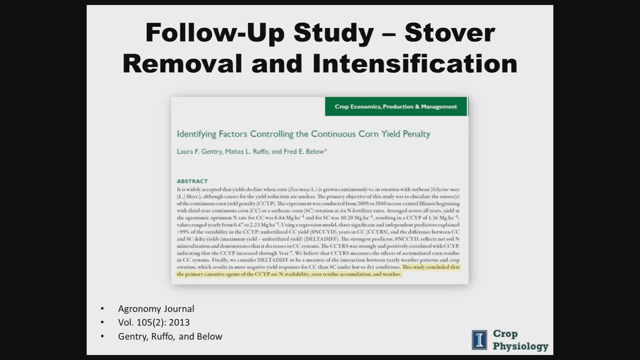 stover, we thought that we could reduce or even eliminate the continuous corn yield. But we know we don't just go in and pull off 50% of the corn stover in a field year after year and not expect there to be some repercussions of that. There are always follow-up effects because everything affects. 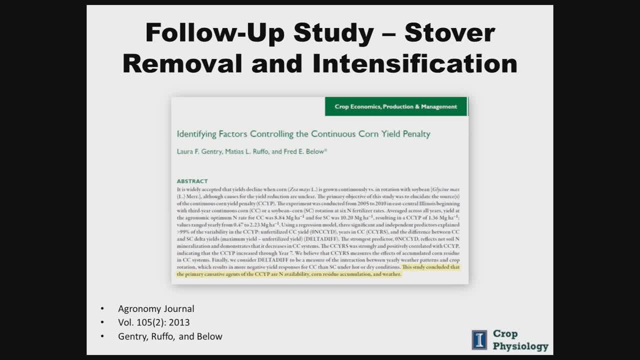 other things in the system. It's all one system, And so the major factors that we were most concerned about were the nutrient availability. When you remove stover, there's a lot of phosphorus and sulfur and zinc in that stover that you're taking off. What is the effect of removing that on the 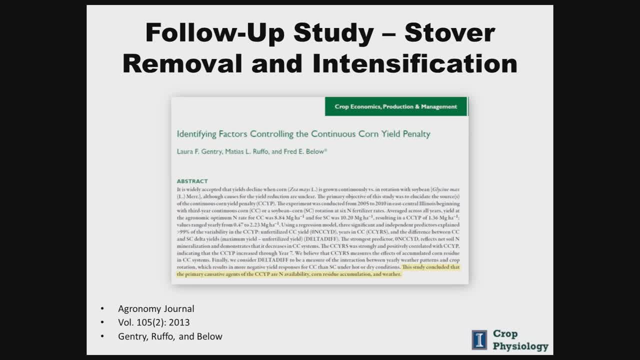 following yield if we don't replace it. And then the second thing we were really concerned about was soil organic matter. We don't want to reduce soil organic matter by removing all of that carbon that's contained in the corn stover. We don't want to reduce soil organic matter to some detrimental 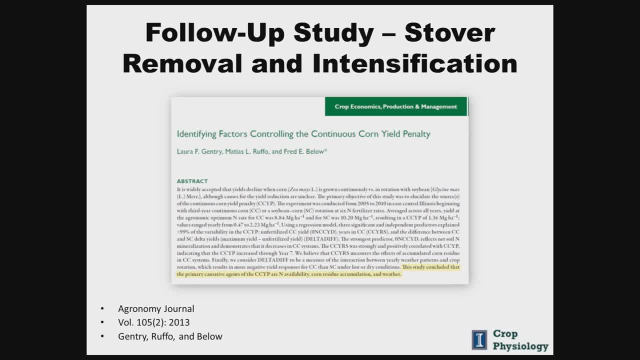 level. So to address that soil organic matter issue, we thought maybe we could increase the plant population in a continuous corn system. What if we increase the plant population which by doing this we hypothesized would increase the root biomass? That's pretty reasonable to think. We thought that on a per acre basis, a higher plant population would have more roots below ground. 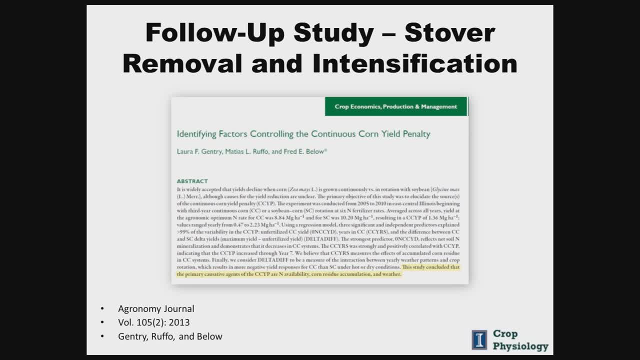 As it turns out, roots are actually a very good carbon source and can build soil organic matter. do build soil organic matter in every system, And so we thought, by increasing the below ground root biomass, we could offset what we're removing above ground with our stover harvest. 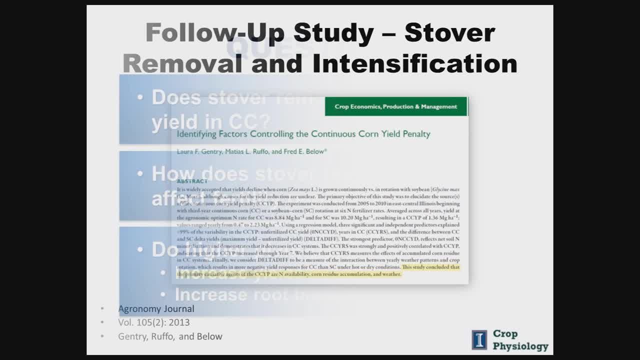 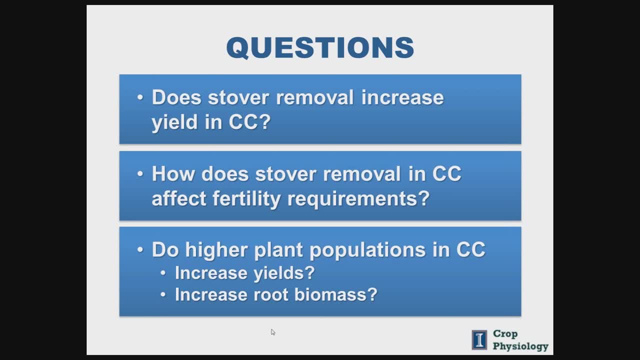 So the questions we were asking in this study were, first of all, does stover removal actually increase our yields in continuous corn systems? And then, second of all, with stover removal, what are we doing to our fertility requirements? Do we need to alter those? and 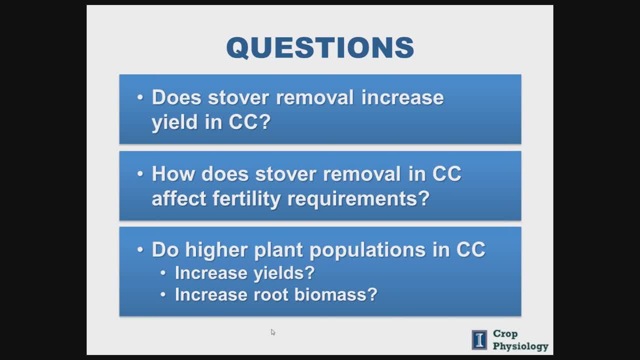 how? And then, lastly, our questions about plant population in continuous corn systems. First of all, can we increase plant populations and will that increase yields? And second of all, will increasing the plant population increase our root biomass? So those were the. 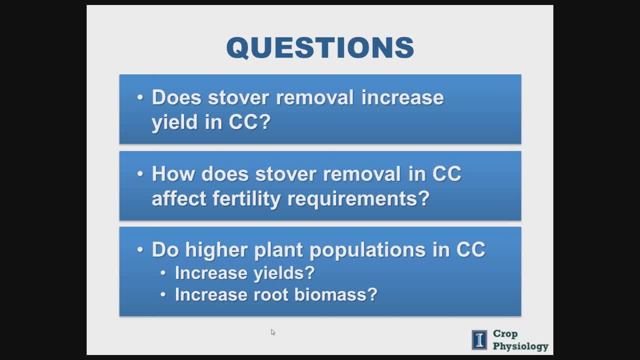 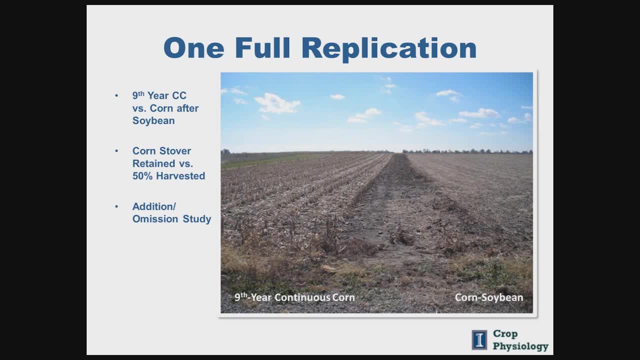 questions that we really wanted to address. Again, this study went right back to the root biomass. So we went back into our previous long-term study, And what I'm showing you here is a picture of one replication of the four full replications that were out there. 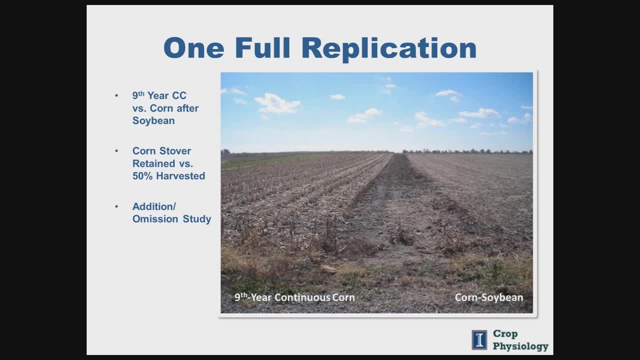 in the field for this study, And so we had one replication, which would consist, first of all, of two large blocks of our rotation crop. So, on the left, what you see is we're getting ready to plant. This is in the spring. We're looking south here And we're getting 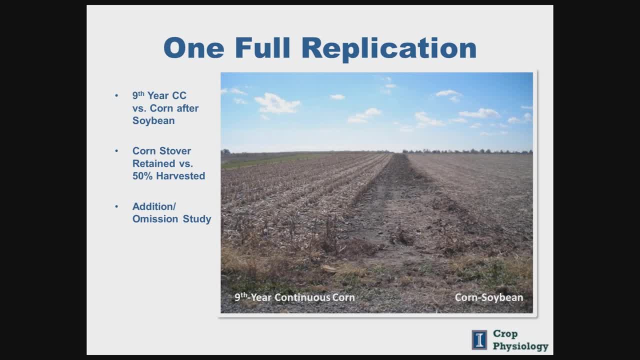 ready to plant our ninth year of continuous corn. So on the left you see eight years of accumulated corn residue. On the right-hand side you see a soybean plot And we're getting ready to plant our long-term corn into our long-term 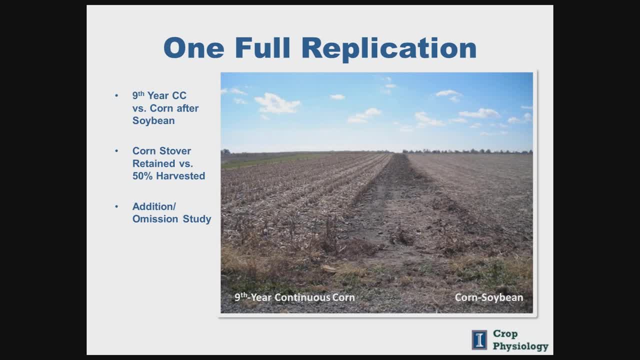 corn following soybean rotations treatment there. Now we wanted to address what happens when we remove 50% of the stover from this. So to do that just in our continuous corn system, because we don't think it's going to be sustainable to remove stover from a 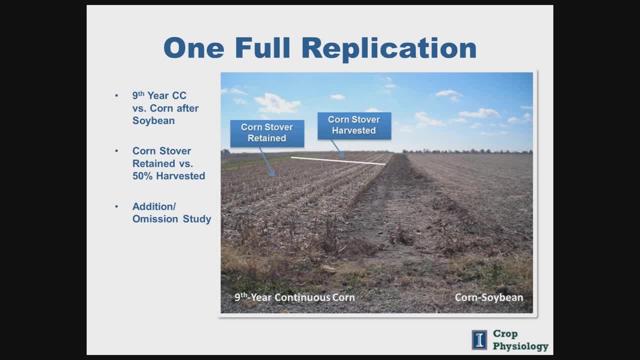 corn soybean system. We take our continuous corn whole plots and we divide those in half, And from one half of it we retain all of the stover And on the other half we remove 50% of the stover. 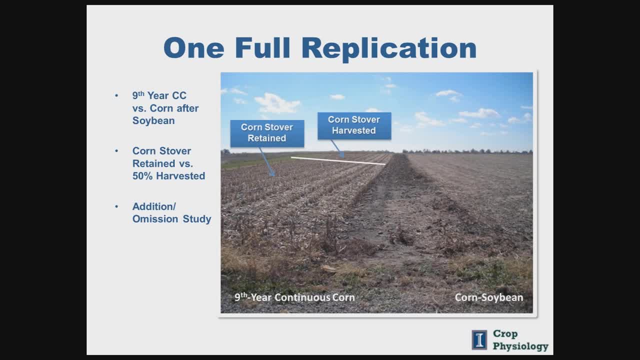 And we do that by flail chopping the whole field. We take off 100% of the stover as much as we can. We weigh all of that And then we replace 50% of it back on the field and we distribute it evenly with a manure spreader. So that addresses our stover removal question. 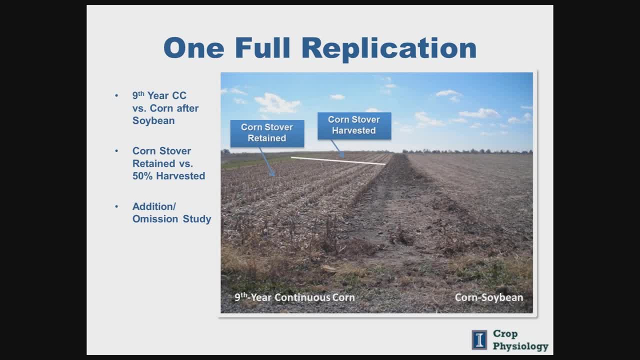 Our last question is what happens in regards to our plant population and our nutrients. To address that, we apply what we call an addition-emission study to each of these larger plots. An addition-emission study is something that we developed here in the Prop Physiology Laboratory. 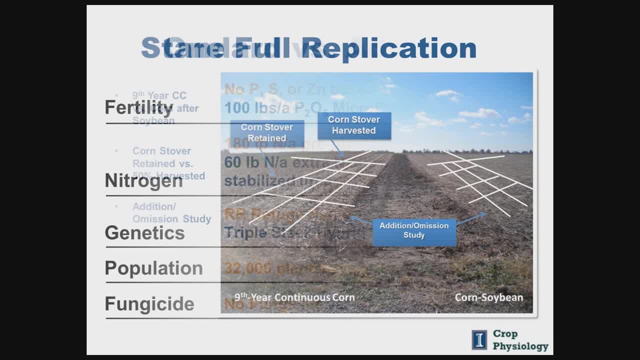 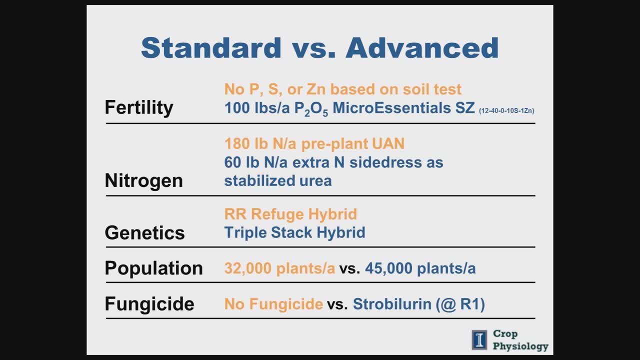 It is a way to address a number of different questions using a fairly limited number of what we call technology factors. In this case, we have five technology factors. Those are fertility, nitrogen, genetics, plant population and fungicide. Each one of those five technology factors is applied at a lower, or what we call a standard level. 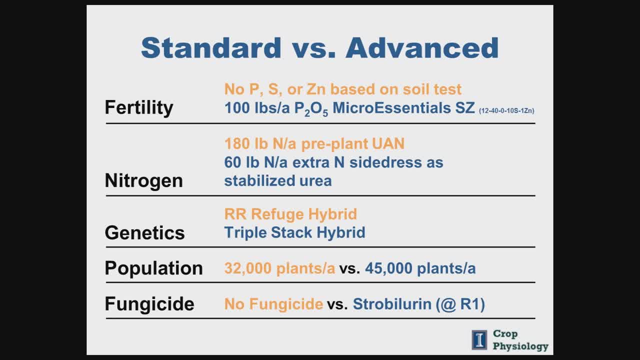 and at a higher, or what we call an advanced level. In this slide, you see, you can see that we're applying all of the lower levels. We're showing that in orange, and then the advanced levels we're showing in blue. For our fertility factor. what we're really talking about is non-nitrogen. 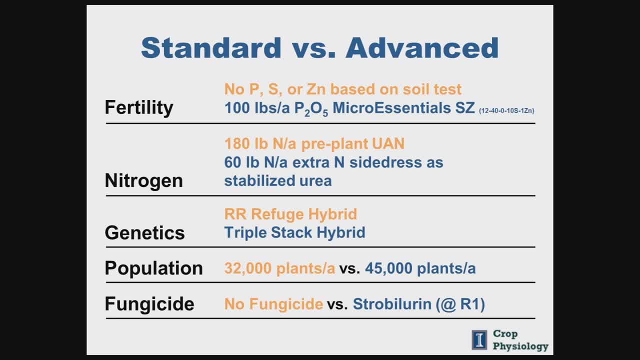 and specifically we're focusing on phosphorus sulfur and zinc, because those are the ones that have our highest harvest index. what we're removing a lot of with the grain We're concerned about those- Our lower or our standard level of that is not to apply any phosphorus, sulfur or zinc. 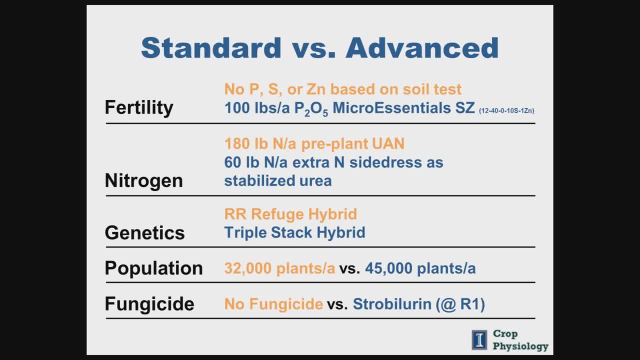 That's based on our soil test recommendations for phosphorus. These were fairly high phosphorus testing soils. The lowest one was about 18 part per million phosphorus using the Bray method. On average, though, it was like 26 part per million. 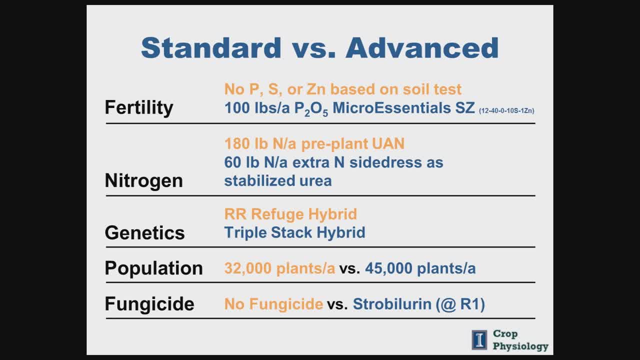 We were not in a range that would necessarily recommend applying more phosphorus to these fields. To look at the advanced level of that, we then applied 100 pounds per acre of a product called MicroEssentials SZ, which is an enhanced MAP product that's produced by Mosaic Fertilizers. 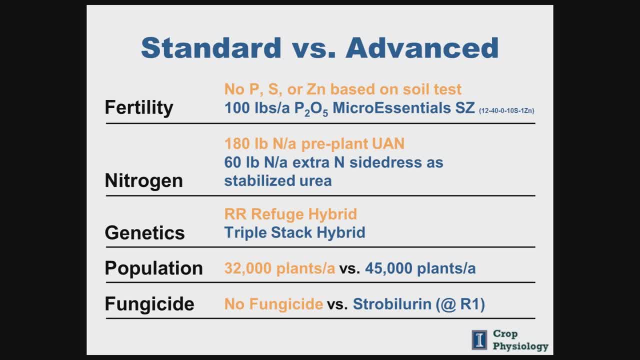 It's got added sulfur and zinc. It's got a formulation of 12,, 40,, 0, 10% sulfur, 1% zinc. To look at our nitrogen technology for that factor, our lower level was 180 pounds of nitrogen applied pre-plant as UAN. 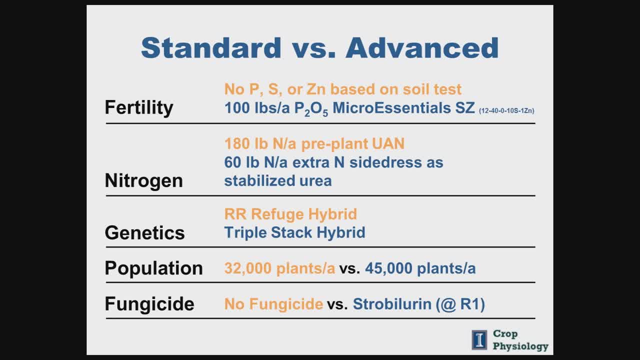 Our advanced level was the same amount applied pre-plant plus an additional 60 pounds of nitrogen applied as a side dress at V5 as a stabilized urea product. Then, in terms of our genetics, we're really talking about insect protection in this case. 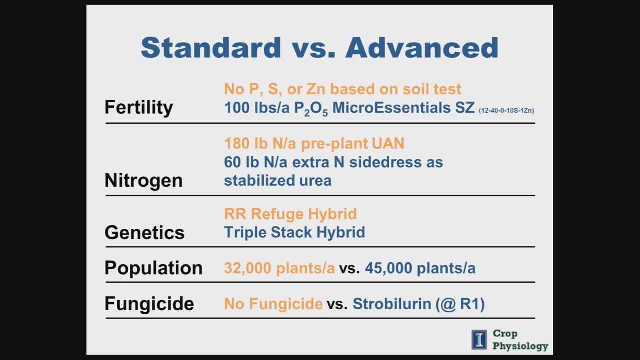 For our standard level of that, we just used a Roundup Ready Refuge hybrid. For our advanced level, we took that same. It was a nitrogen hybrid but with the triple-stack corn borer and corn rootworm protection. That was the triple-stack hybrid. 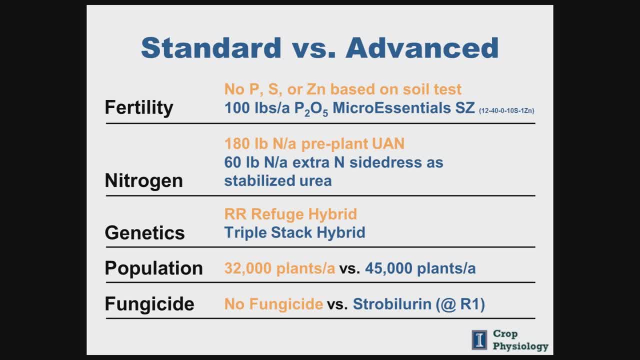 For our plant population it was just 32,000 plants, or 45,000 plants per acre was our lower and our higher level. Then, finally, our fungicide technology factor was, for our lower level, no fungicide versus a strobilurin-containing product that we applied as silvink. 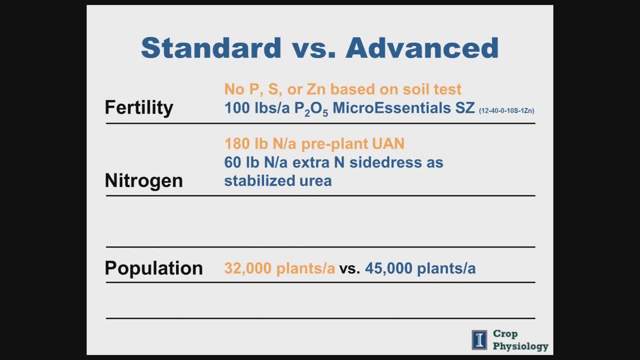 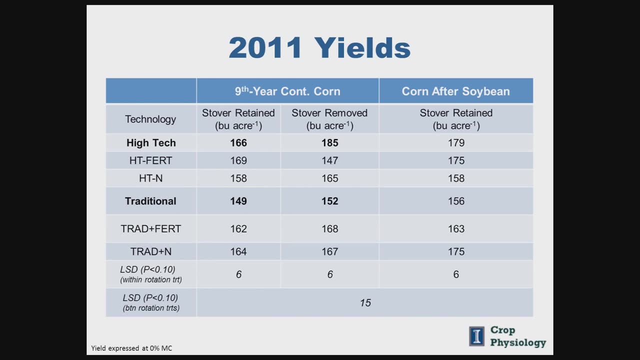 Those are our five technology factors. Today, because of our interest in polytomy, we're just going to look primarily at our fertility, our phosphorus, sulfur and zinc, our nitrogen and our plant populations. Let's look right at our yields. We can begin with our 2011 yields. 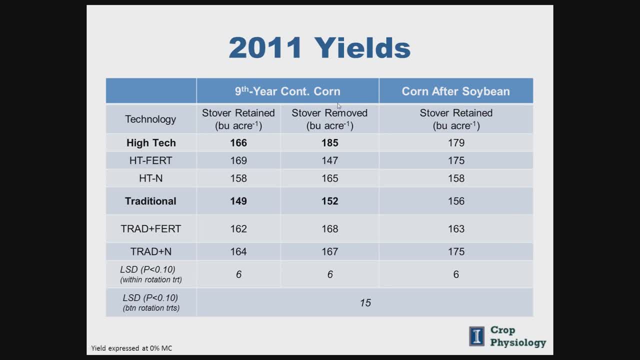 What I want you to look at here, please, is: first of all, we're showing our ninth-year continuous corn treatment, That's both with all the stover retained here and with all the stover removed here on the right. Then we follow that up with our corn following. 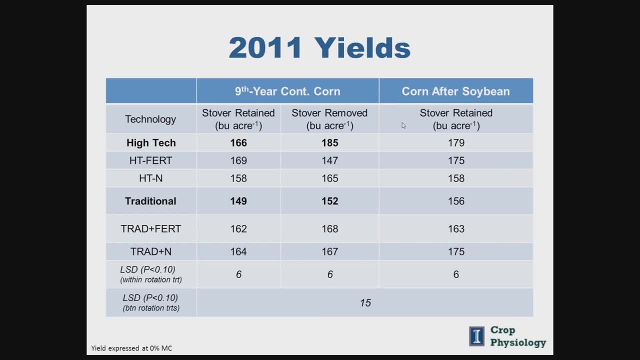 Soybean yields. so you can see, are we overcoming the continuous corn yield penalty? How do these values compare to corn following a soybean crop? Of course, all the stover was retained for that because we didn't have a stover removal treatment there. 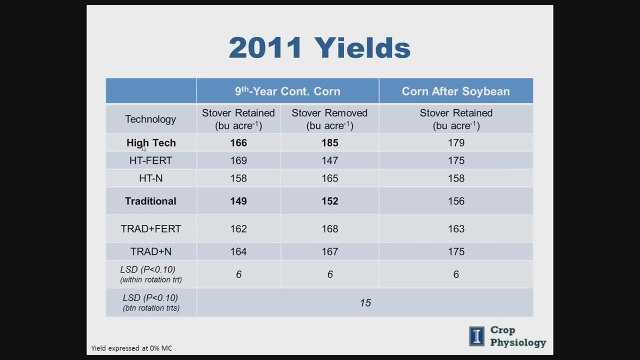 Now you'll see we have these technology treatments. These are just various combinations of those technology factors that I was just showing you. The high-tech technology treatment consists of all five of those technology factors applied at the advanced level. You have higher plant populations, the additional 60-pail nitrogen-cidrus application. 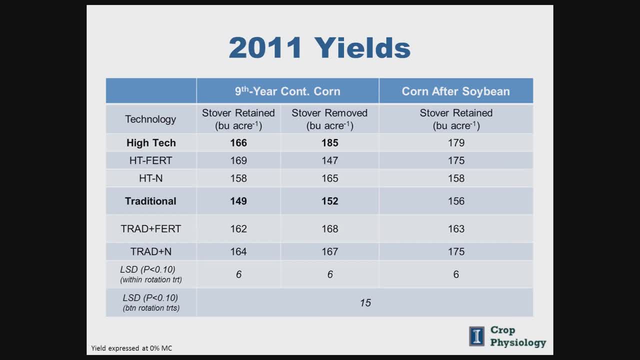 you have the phosphorus-sulfur-zinc application, the rootworm-corn-borer-protected hybrid and the strobilurin product. All five of them apply to the advanced level, The high-tech minus fertility treatment. here that you see is the high-tech treatment. 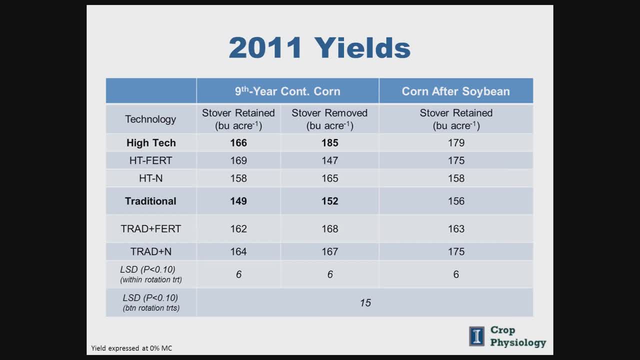 but we just omit the phosphorus-sulfur-zinc application. Everything else is at the advanced level, except we don't apply phosphorus-sulfur-zinc. The high-tech minus fertility treatment is the high-tech minus fertility treatment, but we just omit the phosphorus-sulfur-zinc application. 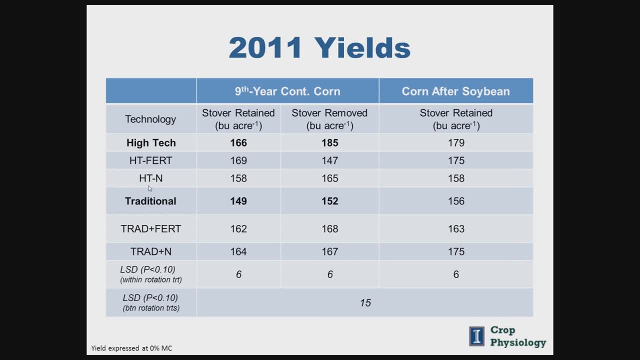 The high-tech minus fertility treatment. again, it's all those high technology factors. So it's the high inputs, the extra phosphorus-sulfur-zinc, all of those except for the additional 60 pounds of nitrogen-cidrus. The traditional technology factor is all five of those technology factors applied at the lower or the standard level. 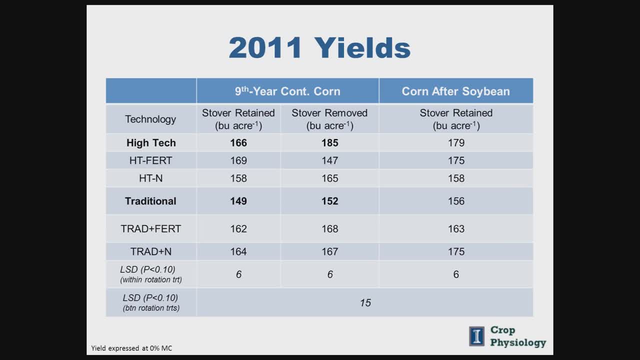 So it's the lower plant populations and no 60-pound-cidrus, no extra phosphorus-sulfur-zinc- the refuge hybrid- and no strobilurin. Likewise, the traditional plus fertility is the traditional treatment plus the additional. 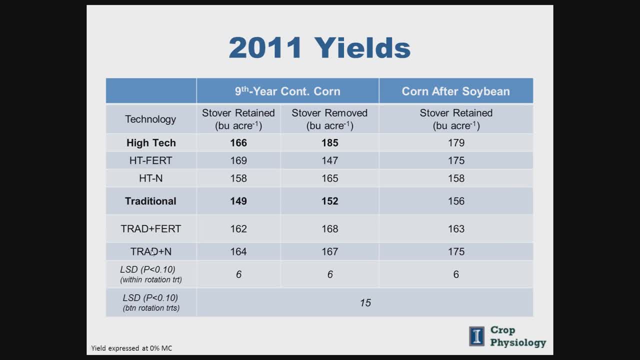 phosphorus, sulfur, zinc, and the trad plus nitrogen is the traditional treatment plus the extra 60 pounds of cidress. So what we are looking at here now are our yields, and the first thing I'd like to take a look at is what happens when we remove 50% of the stover from the system. 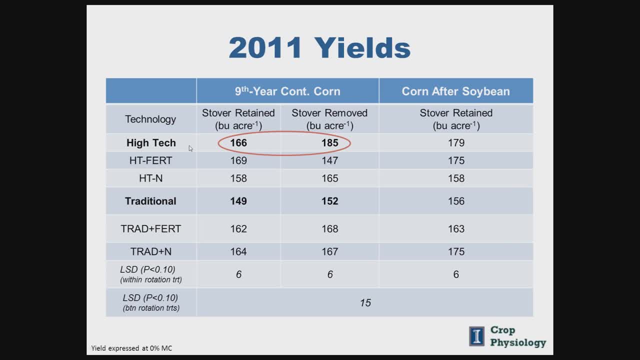 Did we get a yield increase? Well, here, in our high-tech treatment, all the additional inputs, in the high plant population, yeah, we got 19 bushels per acre additional yield, so that was very encouraging. And then I'd also like to point out here that we actually, by removing the additional 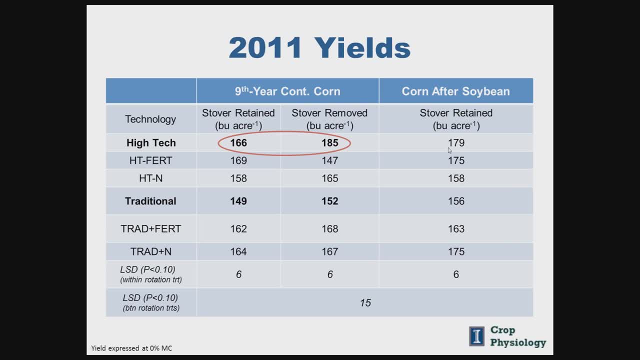 stover- that 50% stover- we overcame the continuous corn yield penalty because we met and exceeded the corn after soybean yields, so that was very encouraging. In the traditional system, though, with our lower inputs and our lower plant population, 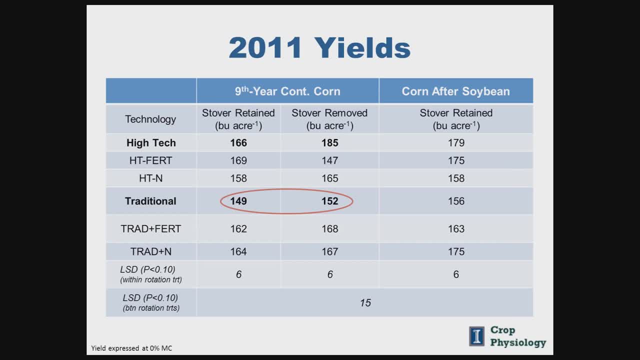 we really didn't get a significant yield increase by removing. So we can conclude that the biggest advantage of stover removal came from that more intensively managed, high plant population, high input system. So let's just focus on that one. So what happened here? when we don't apply that additional phosphorus, sulfur and zinc? 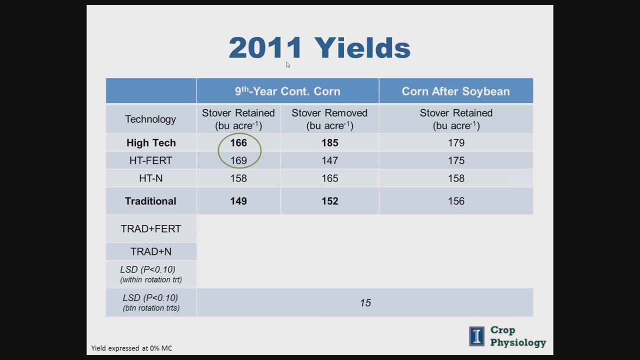 application, when we omit the phosphorus, sulfur and zinc, but the stover is retained. nothing significant happened really. We did not lose or gain a significant output. We did not lose that amount of yield as a result of that. but let's look at what happens. 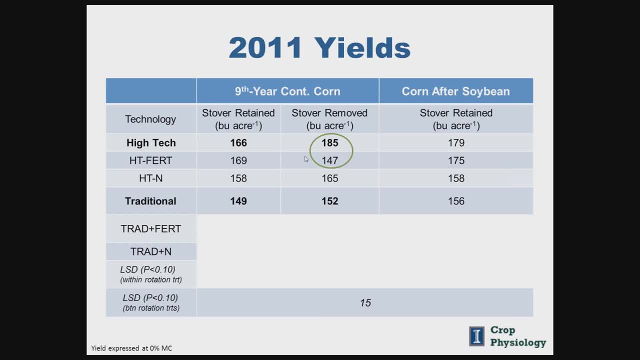 here, when we don't apply the additional phosphorus, sulfur and zinc, and the stover was removed. We lost 38 bushels per acre. This was by far the most significant yield reduction in this system and this really speaks to the value of that stover for, as it degrades and decomposes, releasing these 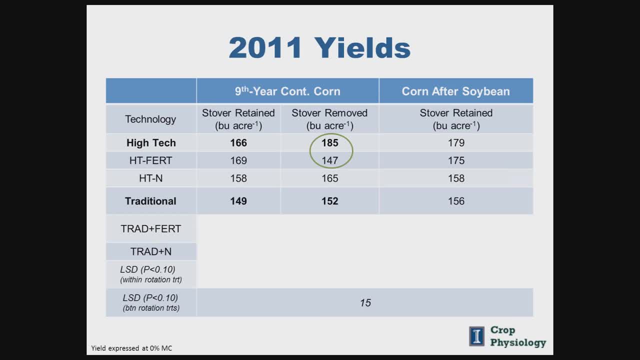 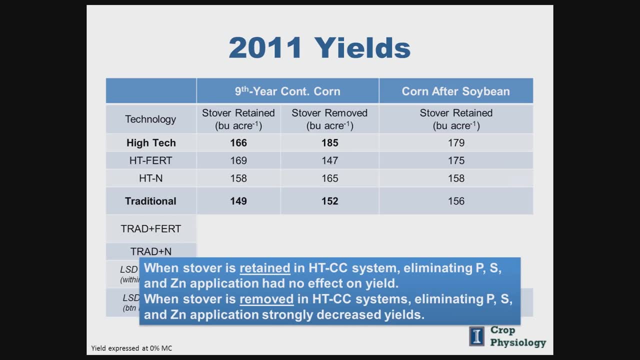 important nutrients. So this tells us you really do need to reapply those nutrients And if you're going to remove the corn stover. So we conclude that when the stover was retained, eliminating phosphorus, sulfur and zinc didn't have a big yield effect. 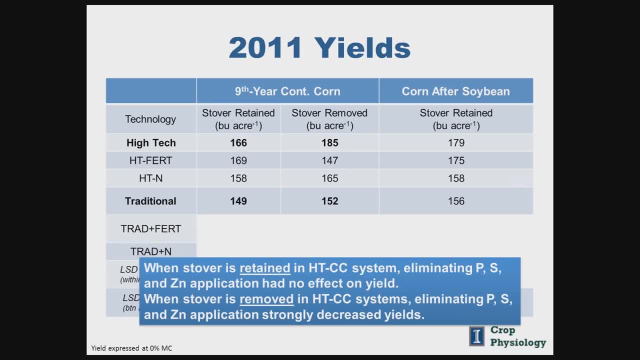 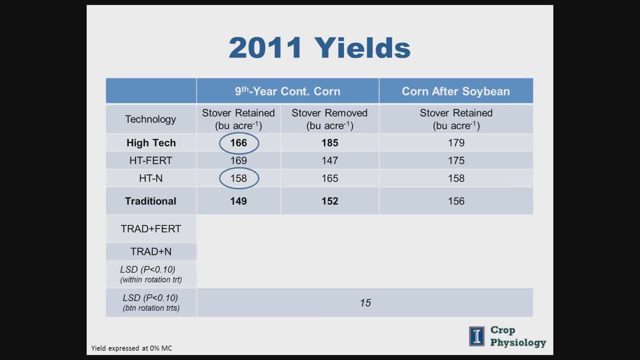 But when the stover was removed and you don't apply the phosphorus, sulfur and zinc, you can expect some very strong yield reductions. Now let's see what happens when we don't apply the additional 60 pounds of nitrogen side dress application. 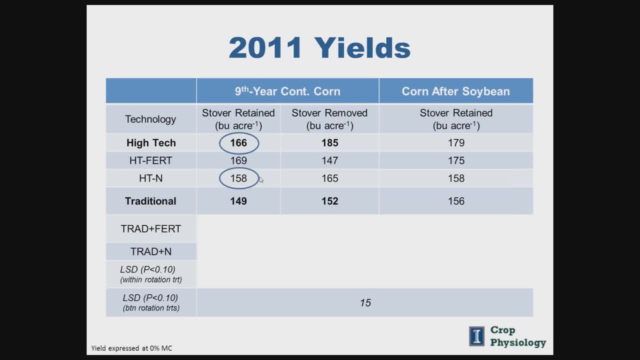 Well, in our continuous corn system, with the stover retained, we did get a significant yield reduction. We did get a significant yield reduction. We lost 8 bushels per acre, but when the stover was removed and we didn't apply the 60 pounds. 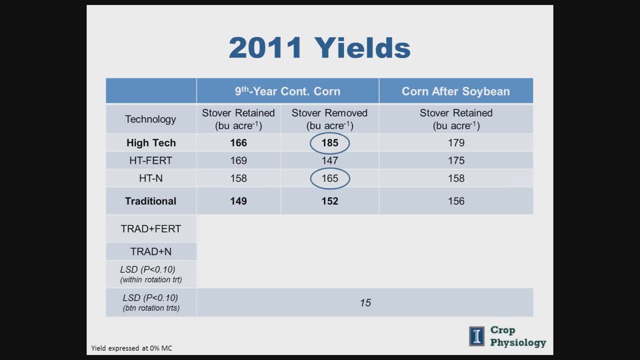 of nitrogen side dress. we lost 20 bushels per acre by not applying it. But the other thing I think is really interesting about this is: I'd like for you to compare, please: the high tech minus nitrogen in the stover removed system: 165 bushels per acre. 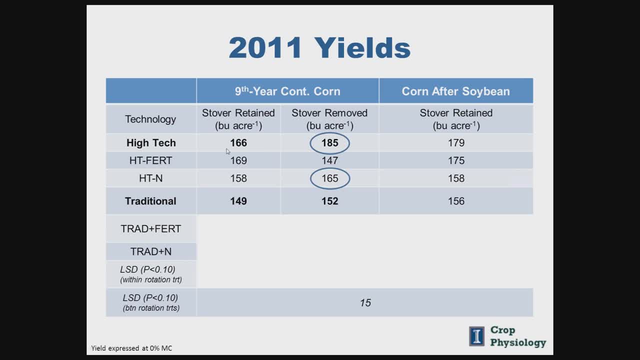 with no 60 pound side dress versus in the stover retained system. So what this is telling us is that by removing our stover, we were essentially giving ourselves a 60 pound per acre nitrogen side dress in that particular year. We wouldn't expect that in every single year, but this is telling us that that stover really 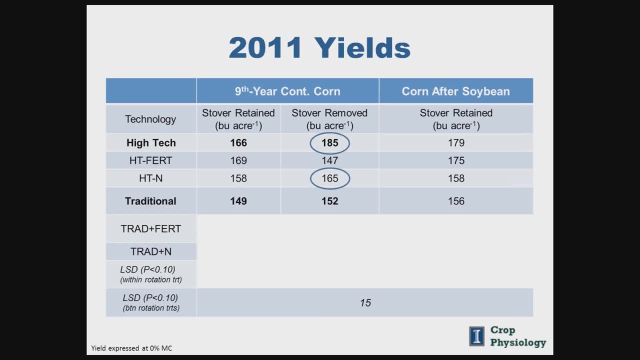 ties up a lot of nitrogen as it's decomposing, And so we do eventually get that nitrogen back. but within that growing season we're losing a lot of the nitrogen. So if we remove some of that stover we don't have to apply the same amount of nitrogen. 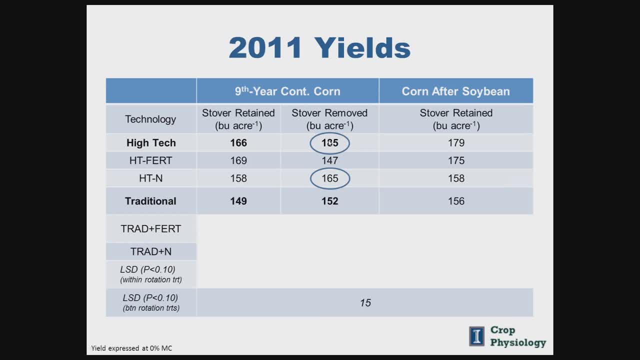 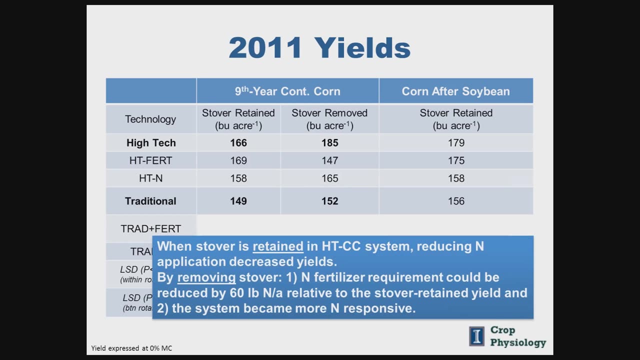 to get the same yields. But if we do apply that 60 pound side dress we get a greater response. We got 20 bushels per acre yield increase in our stover removed system. So this is telling us two things. First, when stover is retained in a high tech continuous corn system, we do lose yields. 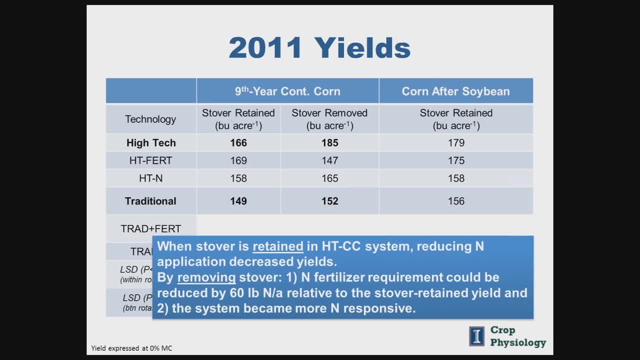 if we don't apply that nitrogen side dress, But if we do remove the stover, two things happen. First of all, we could reduce our nitrogen fertilizer requirement essentially by 60 pounds per acre and get the same yields we would have if we retained the stover. 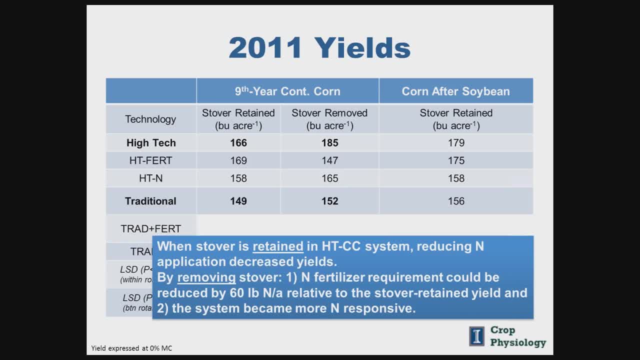 And second of all, the system became a lot more nitrogen responsive. So if in a stover removed system you apply that side dress application, you'll get a greater yield increase than you would if your stover was retained. Again, it's just talking about how much nitrogen is being immobilized by that stover. 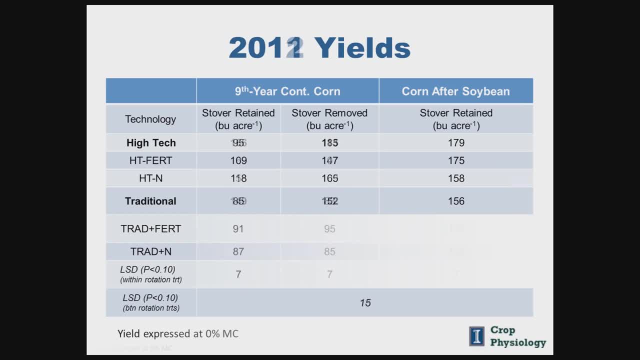 Okay, All right. So now let's look at our 2012 yields just quickly, Because, if you'll recall- and I don't think any of us can forget- 2012 was a dramatic drought throughout all of the corn belt And we had strong, strong yield reductions. 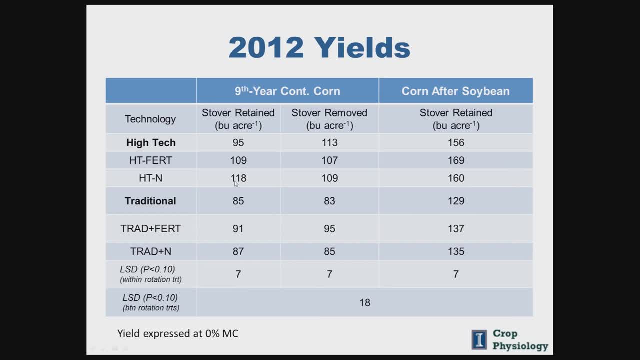 And I think, though, what's really interesting about this is how much more of a yield reduction we got in a terrible drought in our continuous corn system. We lost on average 54 bushels per acre in our continuous corn relative up to our corn following soybean across all of our field trials in 2012.. 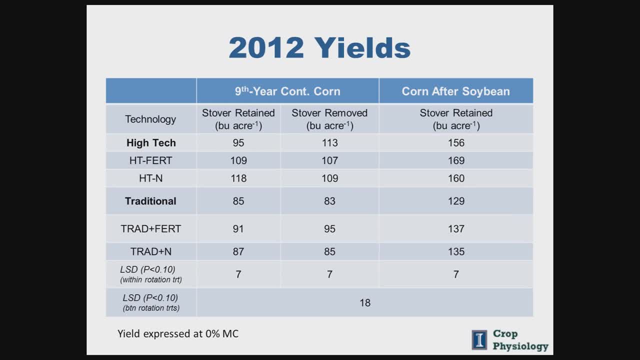 So this actually really reinforces what we found in our previous study, in the paper where we published our model and we said that weather, especially bad weather, has a more significant effect in continuous corn than in corn following soybeans. Corn, after beans, is just a more resilient system. 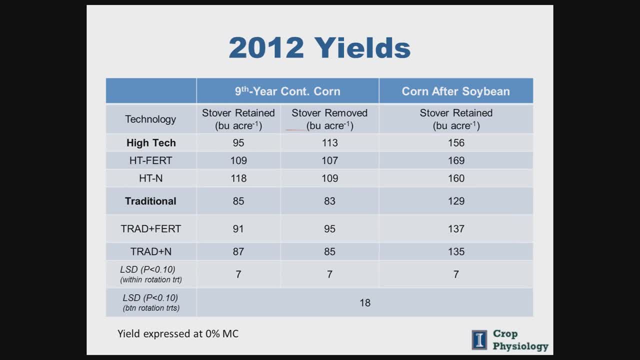 So let's just take a look, though, at what happens when we remove the stover in our continuous corn system in a drought. This was very interesting. This was very interesting. I thought We still got an 18 bushel per acre yield increase by removing the stover, even in a terrible drought. 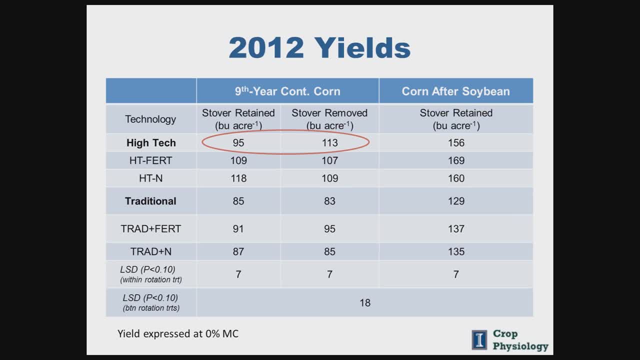 If you recall, in 2011, we got a 19 bushel per acre yield increase, So we are essentially getting the same yield advantage from removing stover even in a bad drought. But you'll also notice, we don't even come close to overcoming the continuous corn yield. 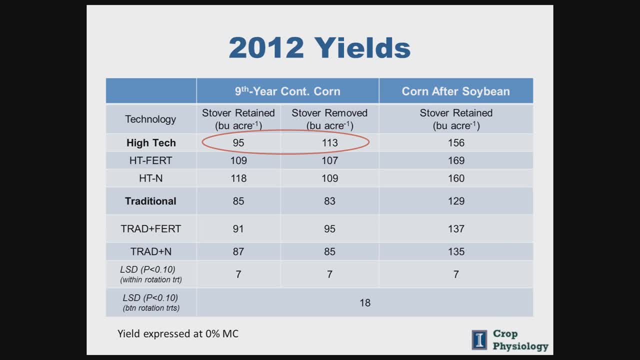 penalty because there's still such a dramatic difference between continuous corn and corn following beans. The other thing In a traditional lower index, Lower input, Lower plant population system, We didn't again, we didn't see that much of a benefit from removing 50% of the stover. 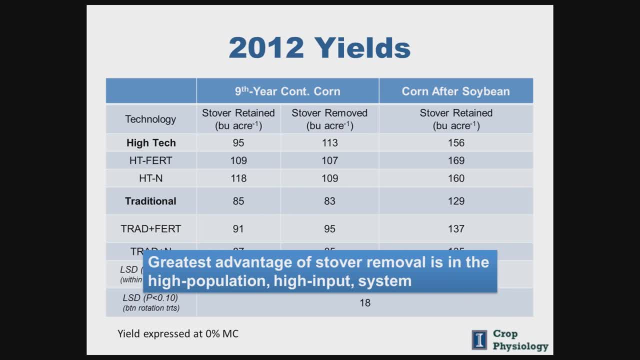 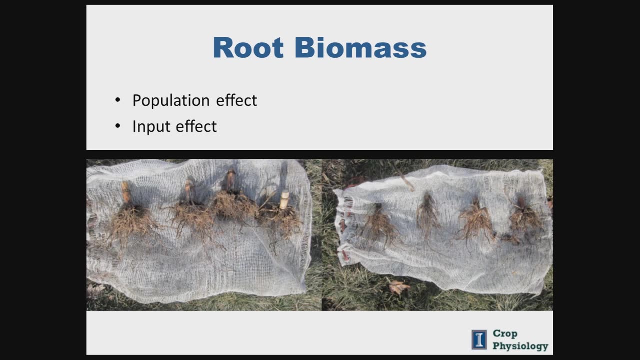 So we conclude that, again, the real advantage of stover removal has to come from this more aggressively managed system. All right, So that's really what I wanted to share about the root yields. So now, if I could, I'd like to talk a little bit about our root biomasses. 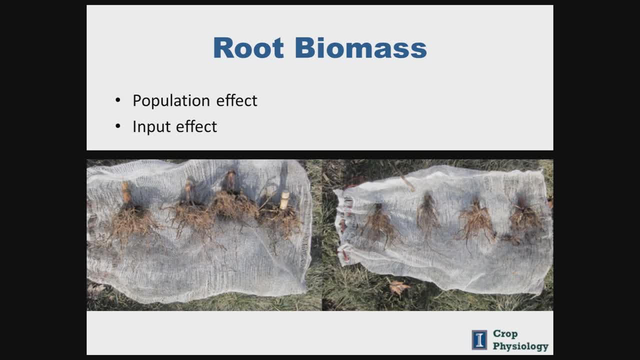 And if you will recall, what we were testing with these- We were looking at our root biomasses- was this hypothesis that if we increase the plant population in continuous corn, we would increase our below ground root biomass on a per acre basis, which we thought would offset some of our stover removal issues, such as reducing 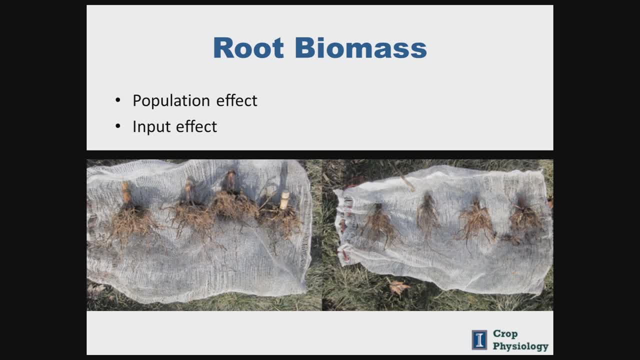 soil, organic matter. Well, what we found was that there was indeed a very strong effect of increasing plant population in continuous corn, but it actually was in the opposite direction of what we had hoped for. When we increased plant populations, we were strongly reduced our per-plant and even our 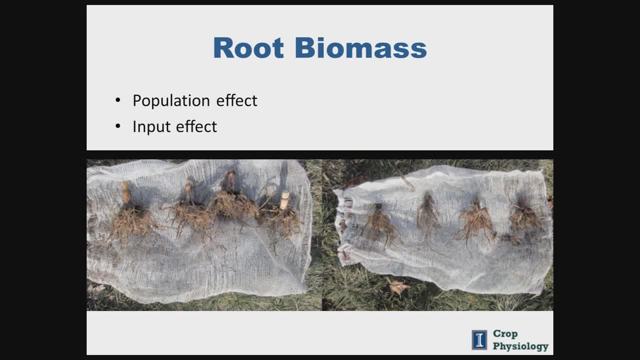 per-acre root biomasses And that effect was actually a lot stronger in continuous corn than it was in corn following soybeans. And then there was another significant effect from the plant populations on our roots, And that was what we found was the input effect. 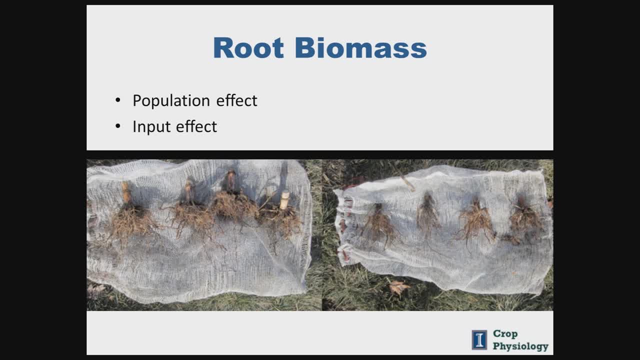 And, in general, what we found was that when we applied more inputs, especially more nutrients, nitrogen, phosphorus, sulfur and zinc had a very positive effect on the root biomass. More inputs meant more root biomass. What we have here is a picture that is a really good demonstration of the typical effect that. 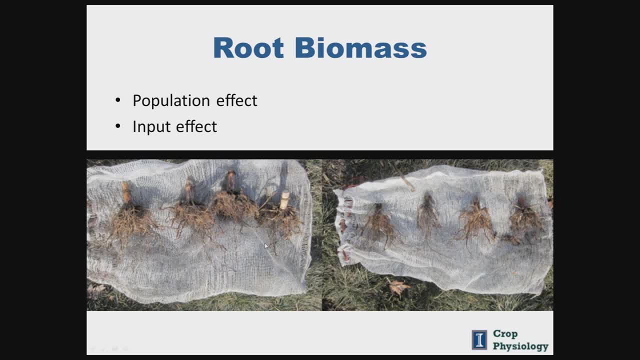 we found from plant populations and inputs On the left-hand side. both of these pictures are from continuous corn plant roots. The left-hand side shows what we saw when we dug the roots from a lower plant population system with advanced inputs: more nutrients On the. 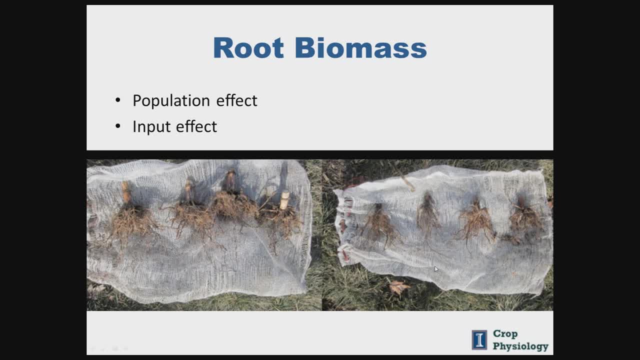 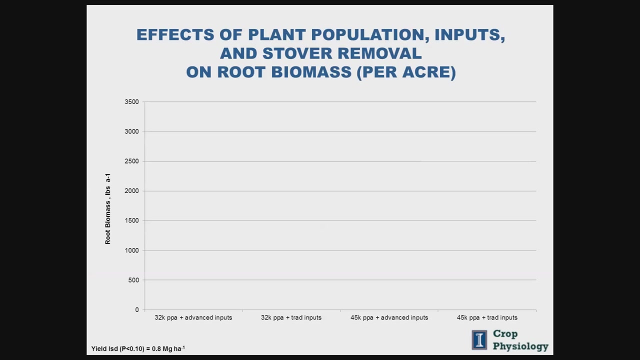 right-hand side. it shows the plant roots from a continuous corn system with higher plant populations and lower crop inputs. You can see it's pretty obvious that there was a strong effect of plant population and input on individual plant roots. What happened on a per acre basis? This is also pretty interesting — it demonstrates the same things that we 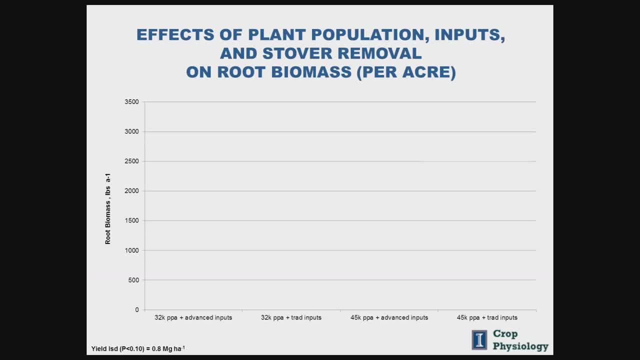 just showed you in the pictures. What I'm gonna show you now is the effects of plant, plant population and crop inputs and stove removal on our per acre root biomasses. So on our vertical axis here we see our root biomasses. It's just showing you how many pounds of roots we have on a per acre basis. 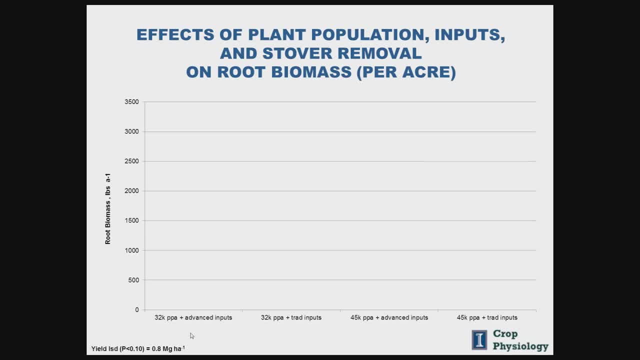 And down here I'm going to show you four different treatments on this horizontal axis. We're showing you the lower plant population with higher levels of nutrients, higher levels of inputs. our lower plant population with our lower levels of inputs. then our higher plant population with our higher levels of inputs and finally, our higher plant population. 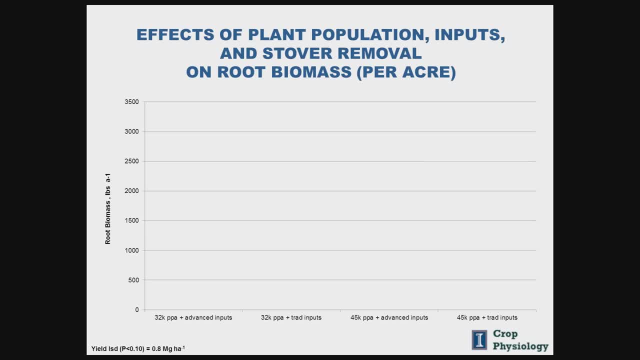 with our lower levels of inputs. So I'd like to first begin by showing you data that is representing the continuous corn root biomasses from our stover retained system. So all the stover was left on here And it's pretty clear what's happening. 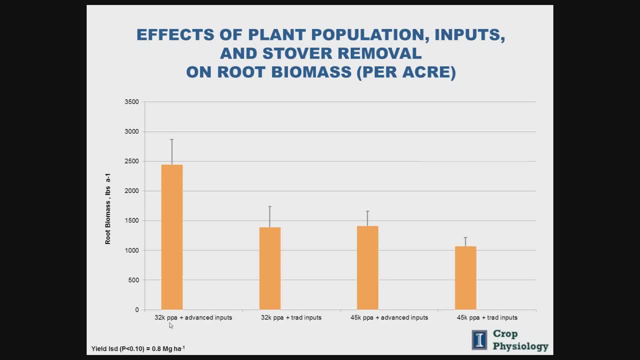 We see that clearly we had the greatest root biomass. We had the lowest root biomass from our lower plant populations and our greater inputs And similarly we had the lowest root biomass from our higher plant populations and our lower crop inputs. And maybe you're thinking: well, that's really fascinating, but what does that mean for crop? 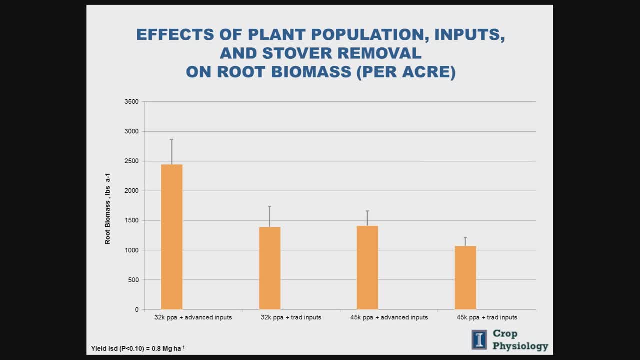 yields. Do more roots mean more yields, Or is the plant producing more roots at the expense of producing grain? So let's just bring in here our yield data, And so I'm just bringing in, I'm just showing you the yields for each one of those respective treatments. 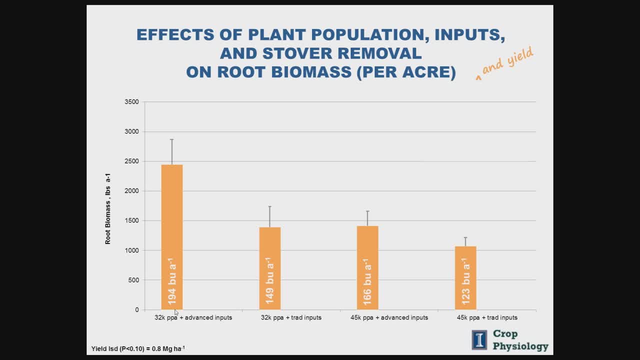 What we see is that the greatest root biomass produced our greatest yields- 194 bushels per acre in this case- And similarly our lowest crop yields came from our lower root biomass. So I thought that was pretty interesting. So that again was our continuous corn system, with all the stover retained. 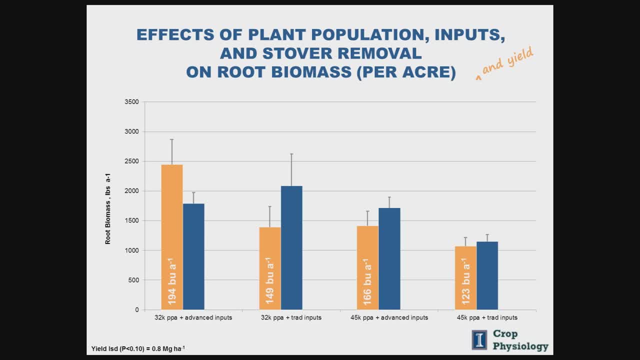 What happens when the stover is removed? Well, it's a little different system. This is continuous corn with stover removed. We see that the greatest root biomass came from the lower plant population, but with the lower levels of inputs. So the question is: did this actually produce the greatest amount of yields? 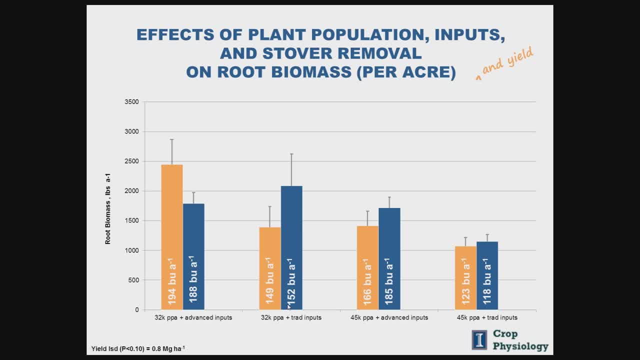 Let's see. No, In this case, this was not the greatest yielding system. Again, the highest yielding system was our lower plant population with higher inputs for continuous corn. What we would suggest is happening here is that the plant is looking for more nutrients. 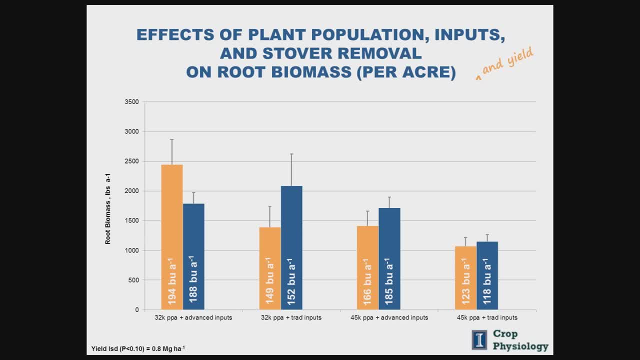 So we're removing 50% of the stover. We're removing a lot of the phosphorus, sulfur, zinc and nitrogen. The plant is sending out greater amounts of roots. It's taking its allocated carbon, putting more roots into the ground to find more nutrients. 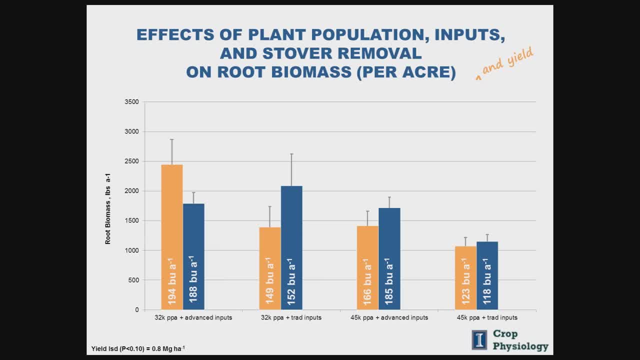 That's at the expense of yield in this case. Then, just as a frame of reference, let's see what happens with our corn following soybean. All I wanted to show you with this is that it's just not as dramatic an effect. The roots, again, are just more resilient to higher plant populations. 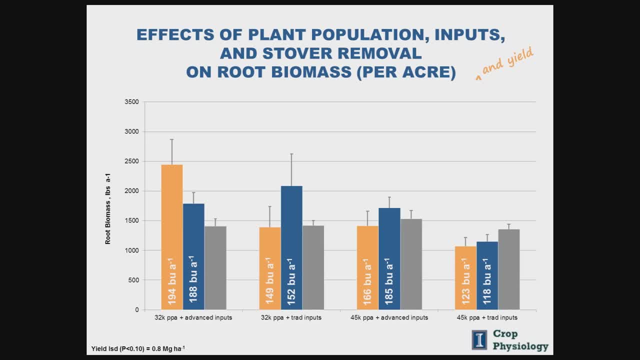 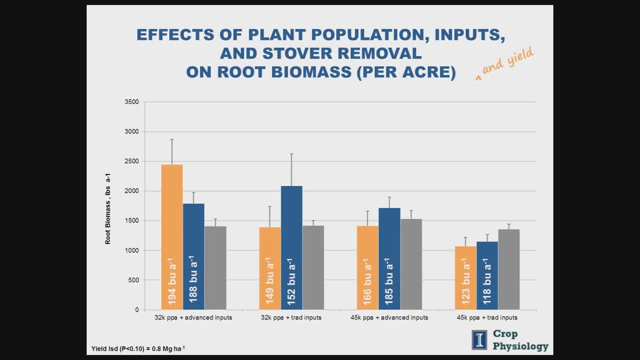 It's growing more and more. It's growing more and more. The roots again are just more resilient to higher plant populations and to lower levels of inputs in a corn-solubing system. The whole system is just a little more resilient. 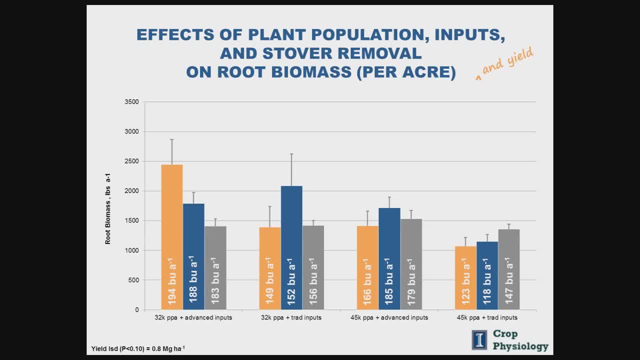 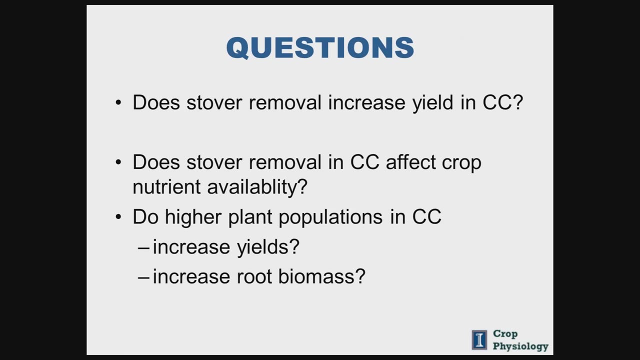 Again, the yields. I think this is really telling us that to optimize yields in a continuous corn system, we might want to consider reducing our plant populations but increasing our levels of inputs, especially if we're going to be removing the stover. Let's just go back to our original questions. 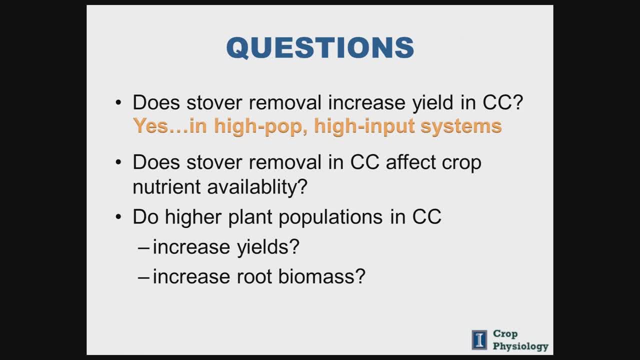 Did stover removal increase yields in continuous corn? Yeah, it really did, but that was really limited to our more aggressively managed, higher plant population, higher input system. Did stover removal in our continuous corn affect nutrient availability? It sure did. It made nitrogen more available and it made phosphorus, sulfur and zinc much less available. 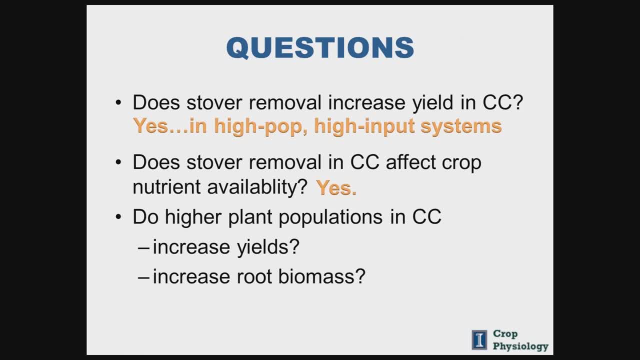 You really need to reapply those nutrients. Then, in terms of our plant populations in continuous corn, did increasing plant population increase yields? No way, Quite the opposite. Did it increase yield? Yes. Did it increase our root biomass? Again, just the opposite. 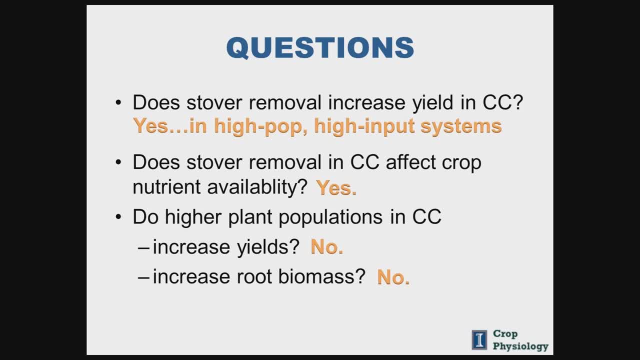 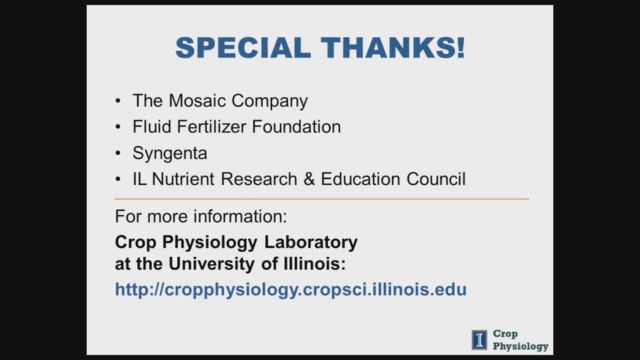 Consider reducing plant populations in a continuous corn system is what this data suggests. We want to thank all of our funders very much. We appreciate their support. You can go to our website here. and finally, I'd like to send out a big thank you to Brian.